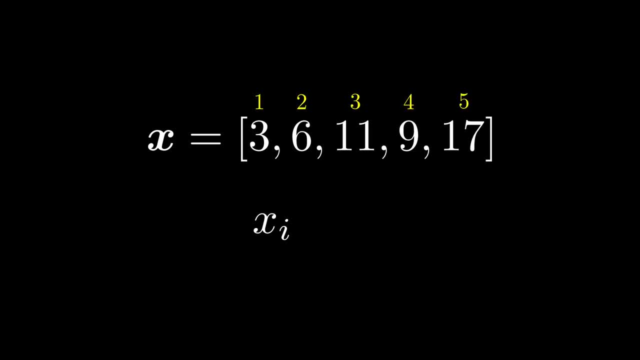 and we can access each of those items in that collection by an index i in a subscript. So x1, x2, x3 can be used to access each of those individual elements in that collection. Note carefully that this uses one-based indexing, not zero-based like a lot of programming languages. 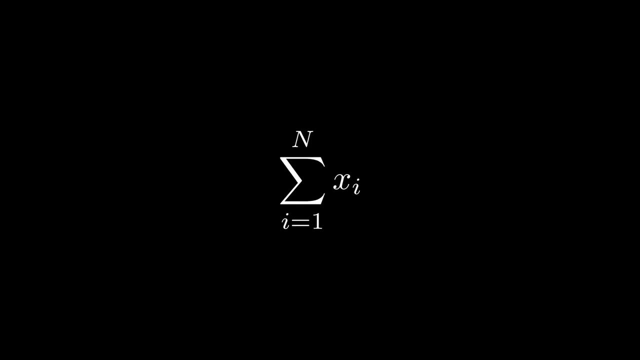 We can apply this logic for summation as well, where we sum elements in a vector or a collection together. So when you see that capital sigma notation, note: we use that index variable i and i is going to be starting at one. the maximum is going to be five. so that's what we change. the 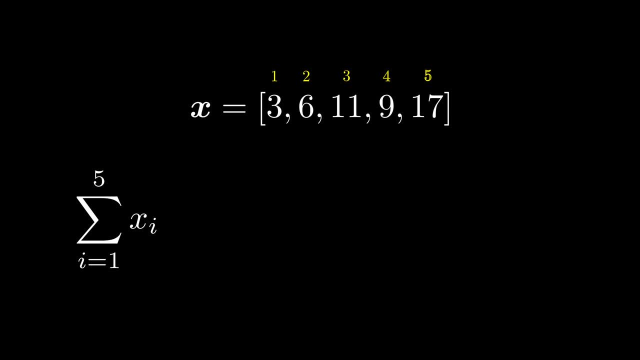 end to and we go and retrieve each of those corresponding elements at those indices between one and five and sum them together. Now let's say we only wanted to sum the middle three elements. What we can do is we can restrict our iteration to only happen between elements of. 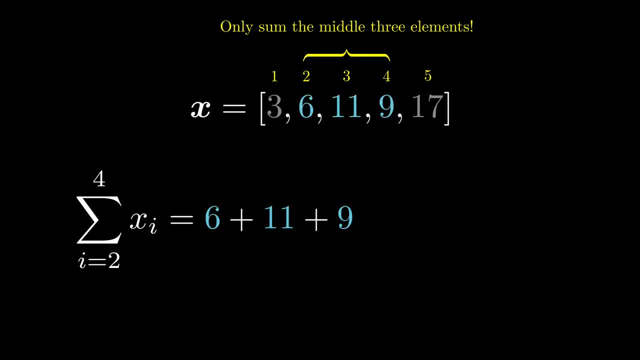 index two through four and add only those three elements together and that would give us a sum of 26.. This demonstrates your summation series does not have to iterate the full collection. Here's another example where we are doing a summation on the expression x squared times x. 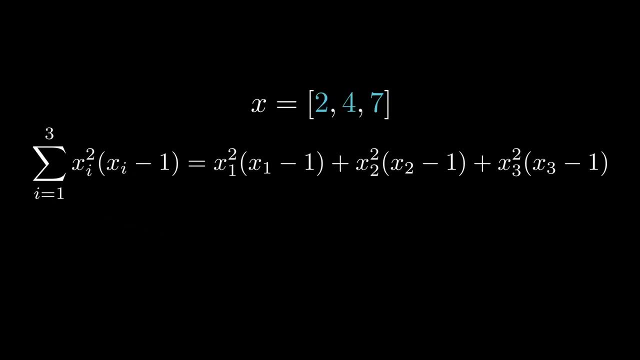 minus one, So each of those x elements we are going to apply to that function and then sum them together. So we plug in the two, we plug in the four, we plug in the seven to that expression and we just simply sum them all together and that'll be 346.. You don't necessarily have to. 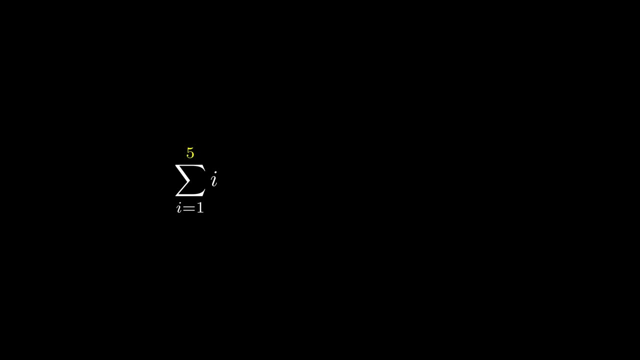 use a summation to work with a collection. You can simply iterate the index variable and sum it together. When performing a summation or a product on the full collection, you can actually implicitly remove the bounds, and that will imply that you're not going to be able to sum the 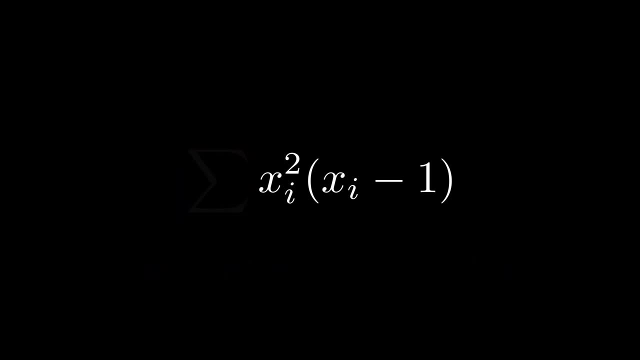 elements together. You are summing all of the elements together. You can actually remove the summation symbol altogether with an index variable like x sub i, and this would be known as Einstein notation. This again would imply a full summation on a collection, A capital. pi works the exact same.